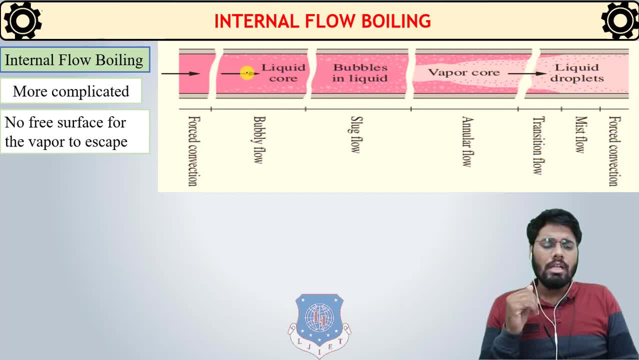 enters at a higher rate In. so this of water is rise After some length. we will see some here. from figure we can see there are some bubbles which is near to the surface of the wall, So this is the zone which is known as the bubbly. 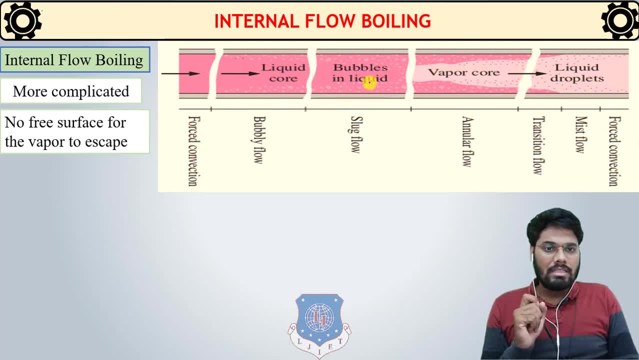 flow. After some length. the position of this bubble is little bit far from the surface of the inner surface of the pipe. So there is a more amount of bubble which is in the liquid which contains vapor in it. So this flow is known as the slug flow, where the number of bubbles is more. 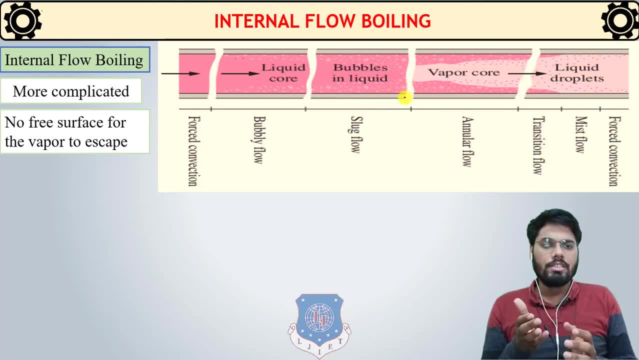 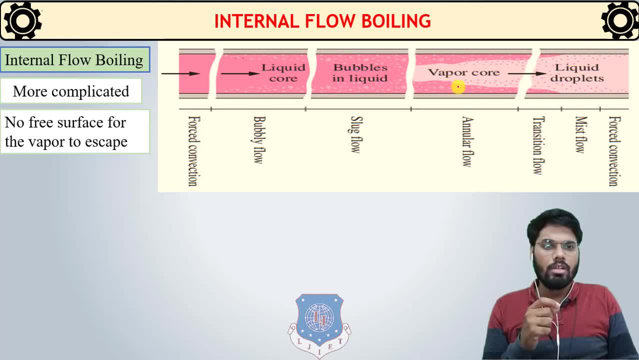 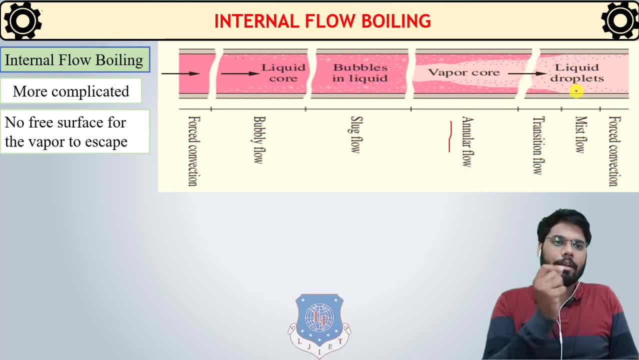 liquid available is only in the bubble form, in the droplets form. As you can see here there are liquid droplets, otherwise it is mostly vapor. so that this is known as the missed flow, where the forced convection, because of the velocity, there is a convection which is done by the forced convection. So this is how internal flow boiling. 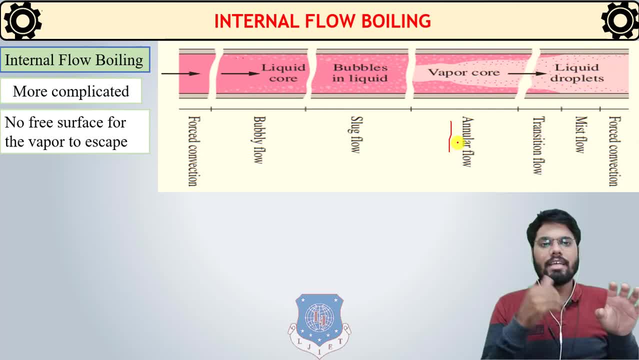 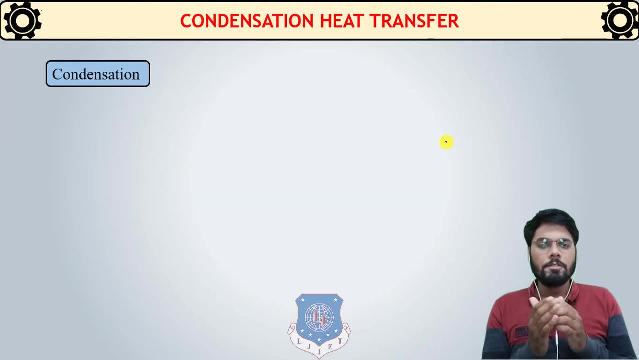 takes place in any pipe in which fluid is flowing by the external arrangement, such like a pumps. External boiling is done over the surface of the cylinder or the pipe, which is nearly same as the pool boiling. Now let us understand condensation. Up to this point we have learned. 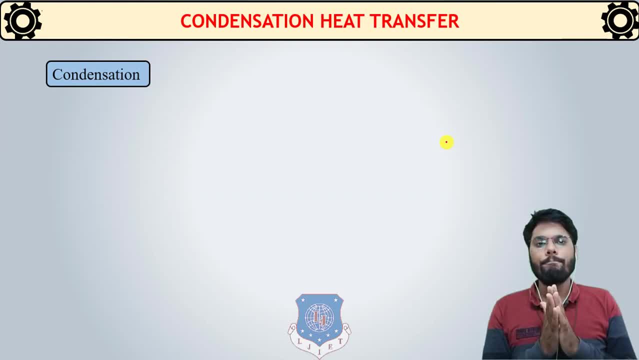 about the boiling process. In boiling, the liquid or the fluid accept or receive the heat from the surrounding latent heat and use that latent heat for the phase change from converting from the liquid to the vapor. This is known as the boiling. It mainly classified in a two ways. First is a 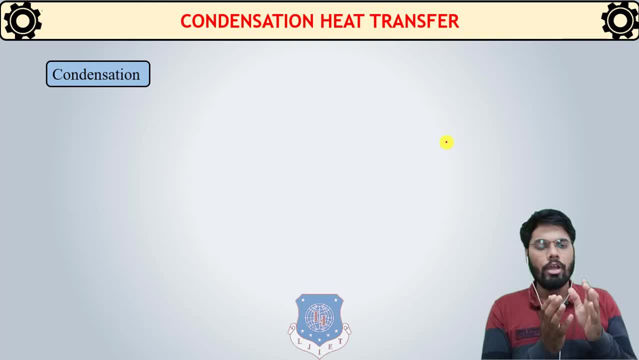 pool boiling. second is a flow boiling. In pool boiling there are also a saturated sub pool boiling and saturated. We have also learned some boiling regimes in our previous video. In a flow boiling there are internal flow boiling and external flow boiling. Basically, internal flow boiling is which is 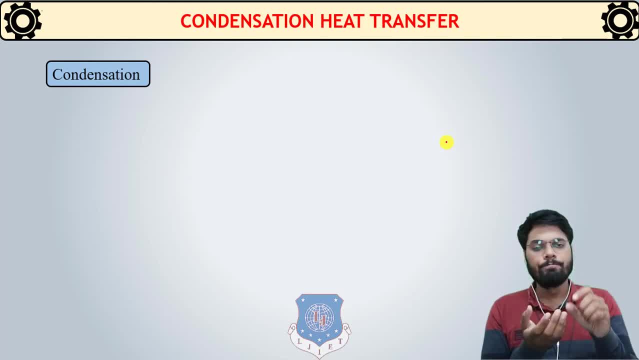 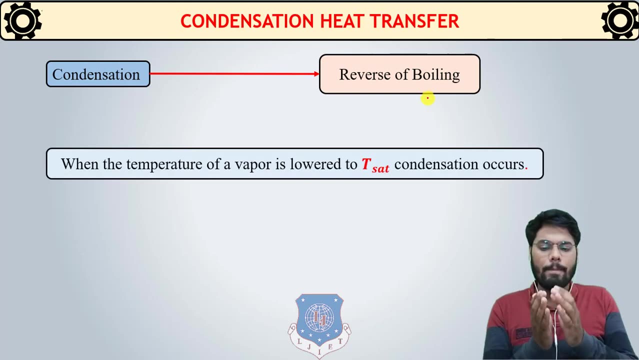 much complicated because in internal flow boiling vapor and the liquid both have to flow inside the pipe. There is no free space available for the vapor to escape. Now it is time to learn condensation. Condensation is just reversal of the boiling, in which, when the temperature of the vapor 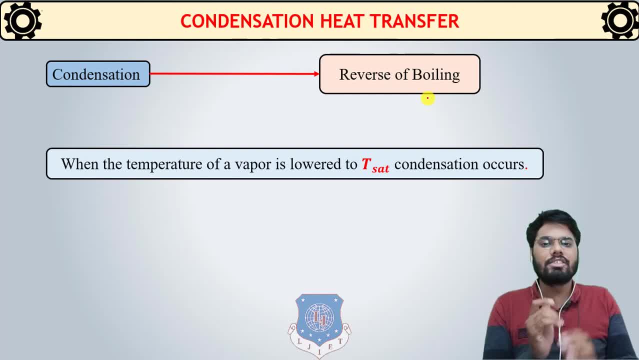 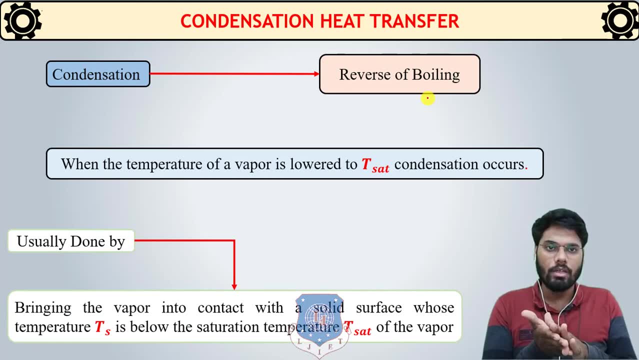 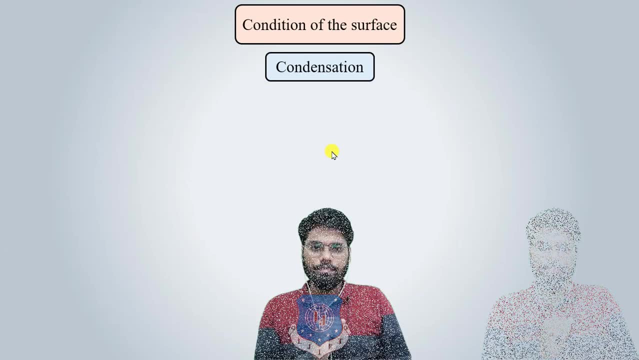 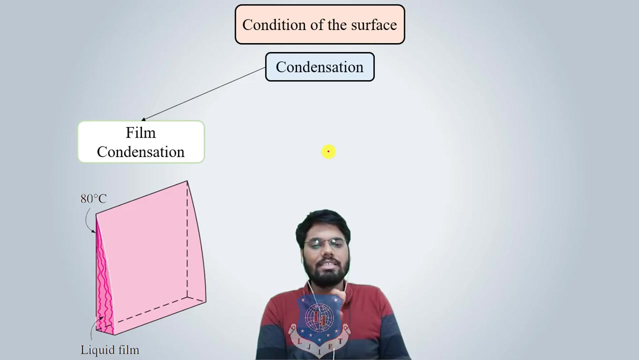 is lower to the saturation temperature, condensation starts. Usually it is done by bringing the vapor into the contact with the solid surface whose temperature TS, whose surface temperature is below the saturation temperature of the vapor. So there are conditions, different conditions for the condensation, According to condition of the surface. the condensation is mainly happens in a two way. 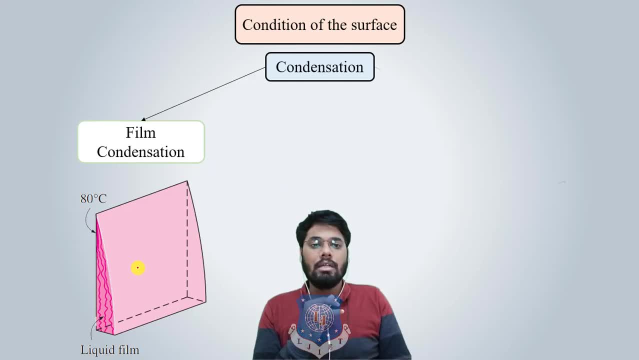 One is the film wise condensation. Second is drop-wise condensation. As you can see from this figure, in a film condensation the vapor condense on the surface and form a liquid layer, or we can say that a form, a film of. 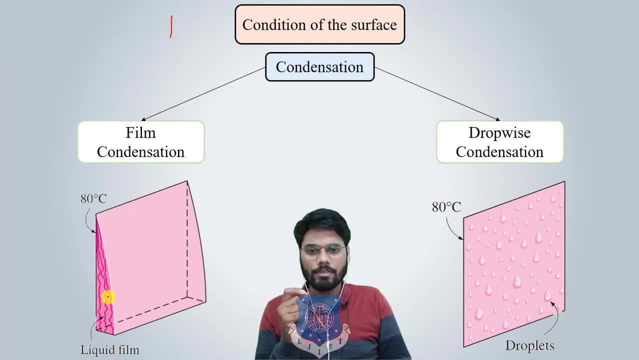 liquid on the surface, of that on the surface. Now, as more content of vapor condense on the surface, the thickness of the film will increase And, due to the effect of the gravity, that film will flow in the downward direction. As we here, we can see that there is a thickness. 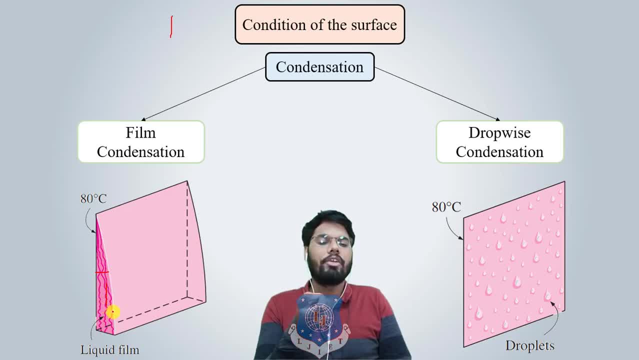 of this film and which is flowing downward direction due to the gravity effect According to condition of the surface. another type of condensation is drop-wise condensation. It is purely depend on the surface condition. In a drop-wise condensation, vapor condense. 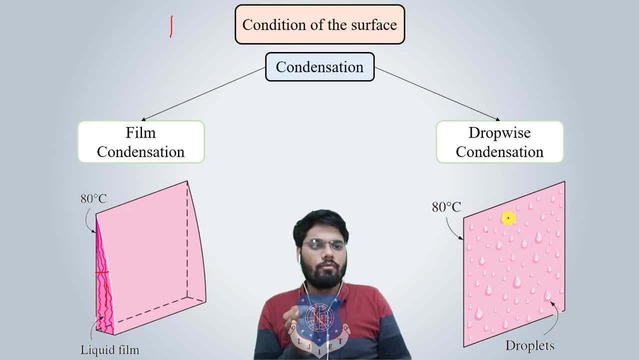 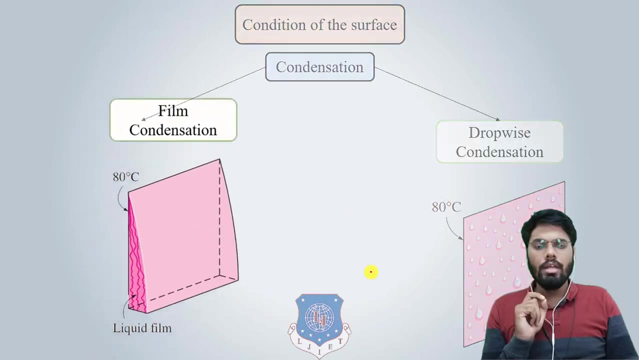 on the surface of the solid in a droplets form. Here you can see in the figure the vapor condense and takes form of liquid in a droplets form. after certain size. this droplets will also flowing downward direction due to the gravity effect. now let us understand both type first.